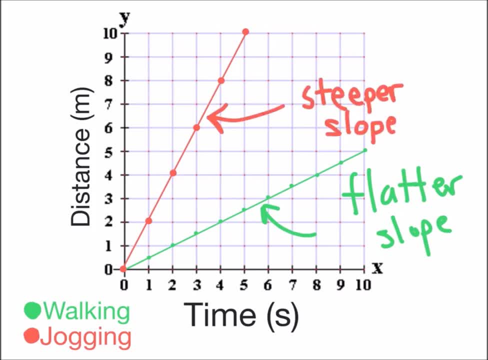 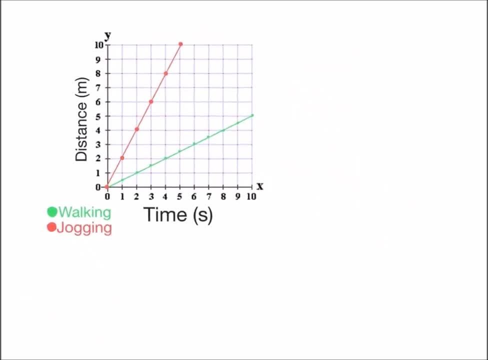 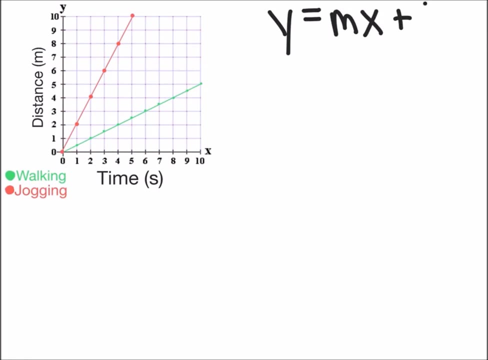 flatter, more horizontal slope, and the red line is a steeper, more upright slope. What we're going to do is compare the speeds of those using numbers To do that. I'm going to move my graph over here. I'm going to look at the y equals mx plus b equation, which is the equation of a straight 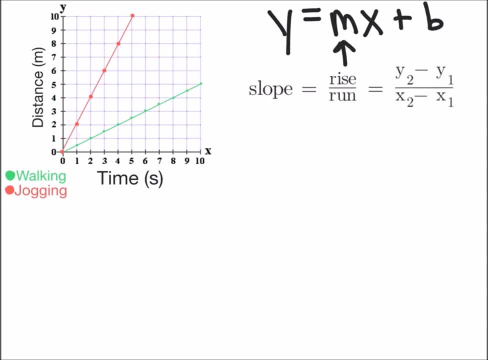 line where the variable m equals the slope, which can be found as the rise divided by the run, or the y2 minus y1 divided by x2 minus x1.. I'm going to use slope equals- rise over run, because I think that's what most of us use, So I'm going to identify that slope equals. 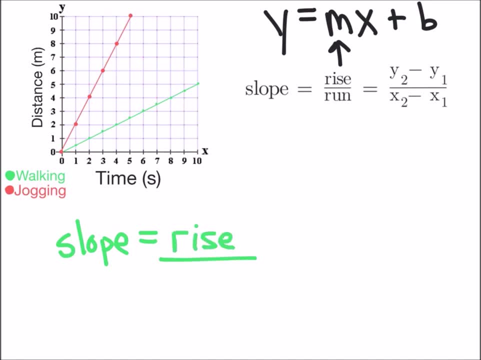 the rise divided by the run. We're going to look at the walking data first. So the rise for the walking data is 5 meters. I'm going to substitute that in for the rise divided by the run, which is going to be 10 seconds Once I do that calculation. 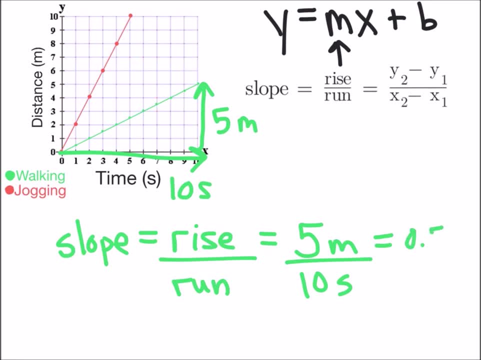 I'm going to get 0.5 meters per second. That's going to represent my speed of the person that is walking. I'm going to write that down just to keep to compare for later. Now we're going to look at the data from jogging. 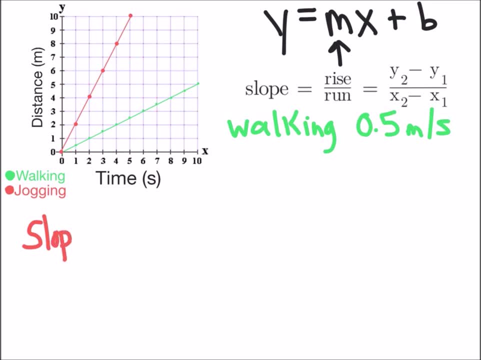 So for that I'm gonna use my slope equals rise divided by the run And look at the slope data for jogging. Here's a slide to look at. OK, For jogging, the rise is 10 meters and we're going to divide that by the run, which is: 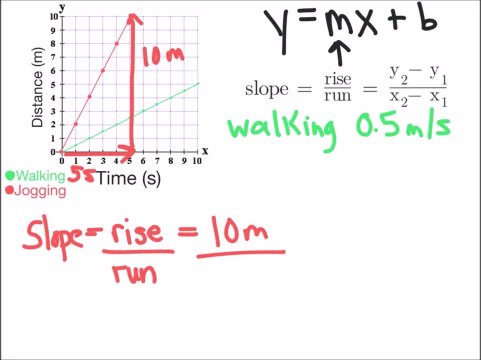 5 seconds and we can do that calculation to get 2 meters per second, which is going to be the speed for the person jogging, And we can compare those two values, the flatter 0.5 meters per second to the more steep 2.5.